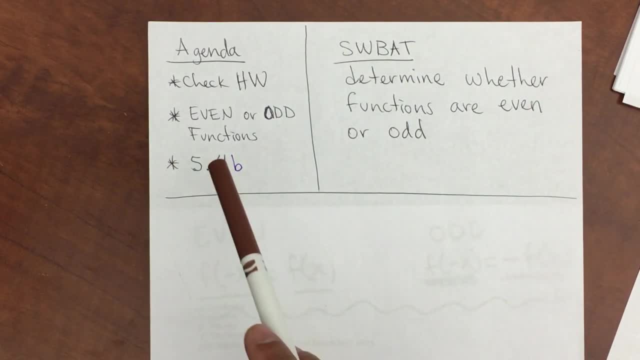 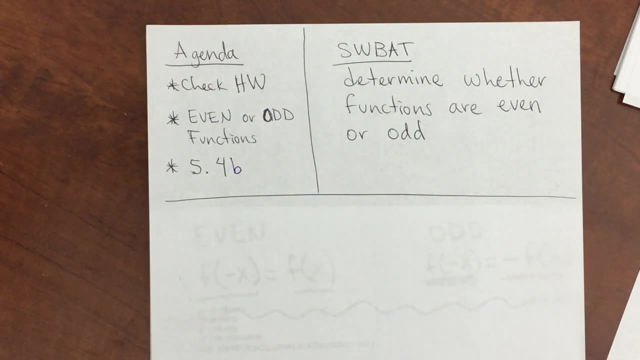 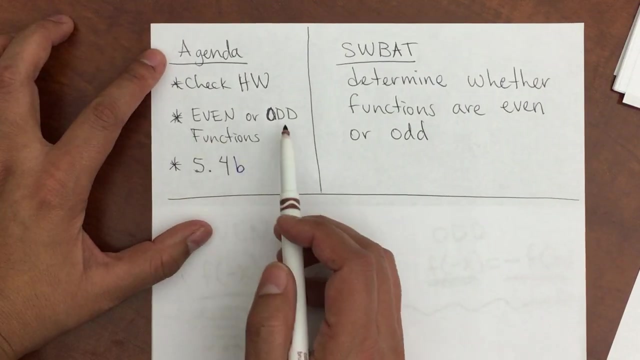 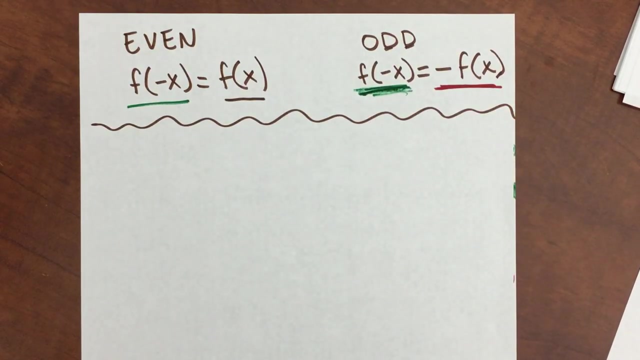 Hello students, today we're going to continue with 5.4b, So it's the same agenda. I just added a b in here because it was going to be a super long video, So I decided to break it in two. But we're going to decide whether functions are even or odd, Okay, whether they have even or odd symmetry, And so, again, these are the formulas that we'll be using to decide whether they are even or odd. 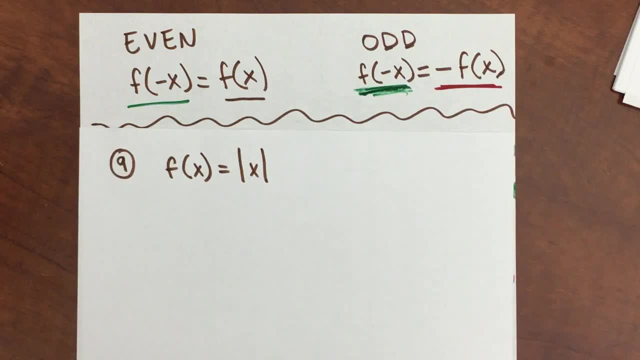 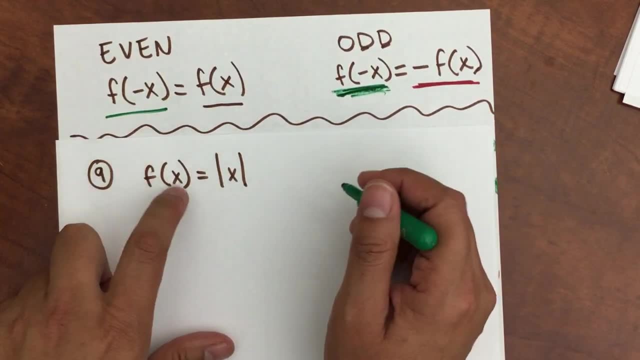 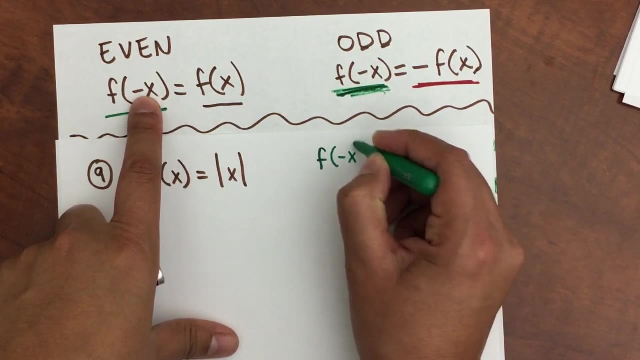 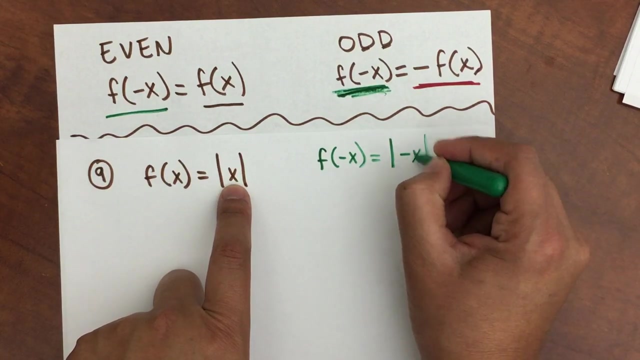 So I have here number 9.. And so, if you recall from the first part of the video is the first- we're going to replace the x by negative x. Okay, so we're going to find the f of negative x by replacing the x by negative x. So in here, what you need to know is that, because of the absolute value, 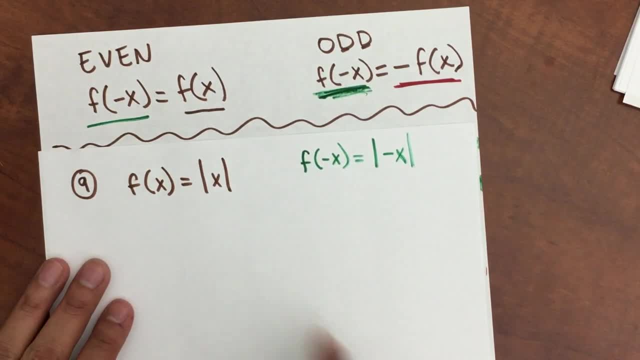 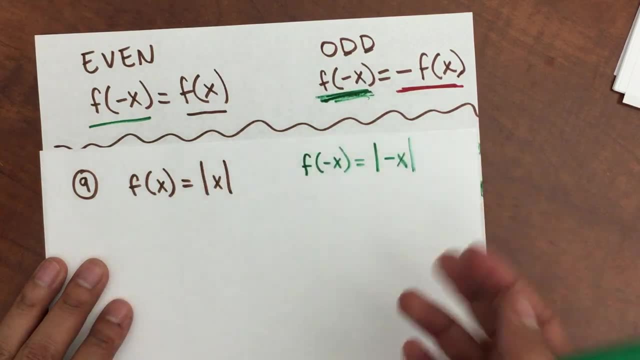 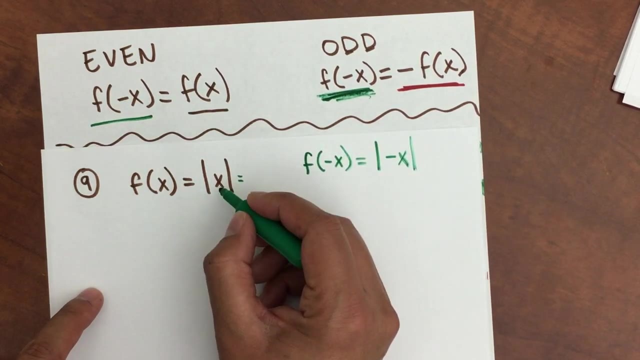 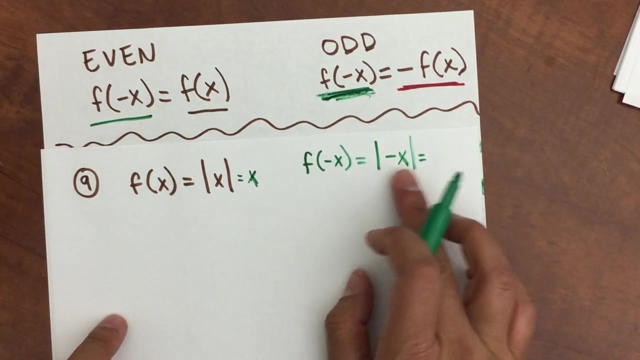 you will always get the same value, whether this is positive or negative. Okay, only if you have one value inside. Okay, if you're adding or subtracting, then that's a different story. So basically, if we were to simplify it, we know that because it's only one value, the answer will always be positive of that x. If we have in here the absolute value of negative x, you also get the positive of that value of x. 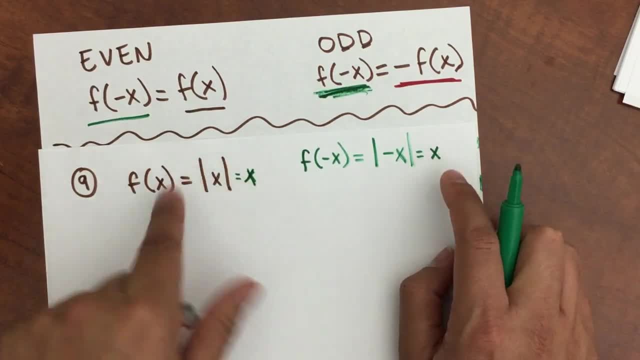 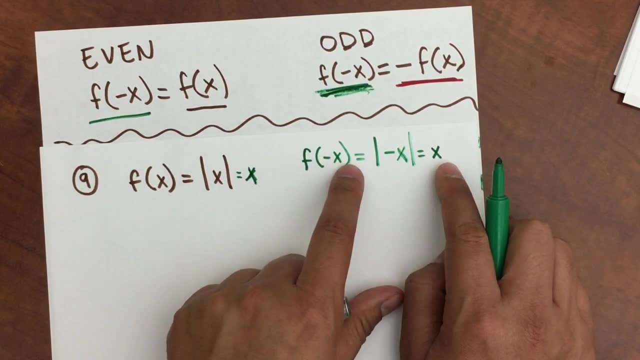 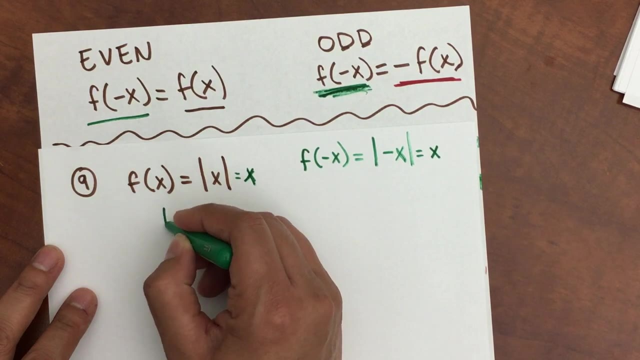 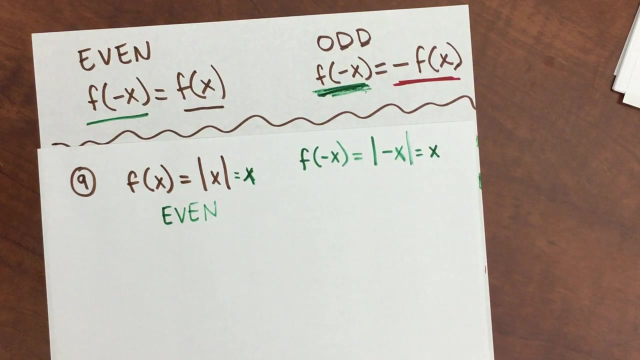 So, again, when the original function is the same as the f of negative 2, I mean f of negative x- then that means that the symmetry is even. Okay, it has even symmetry if they are the same. So I'm going to sketch the graph in here. 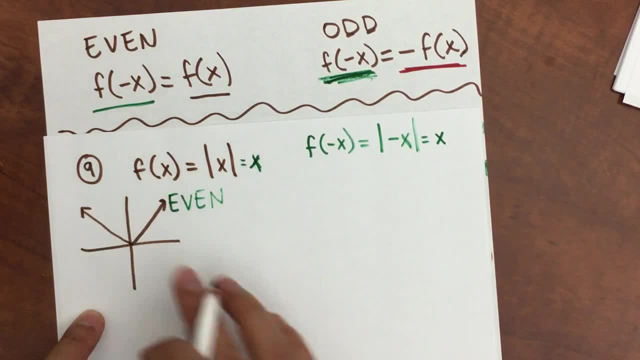 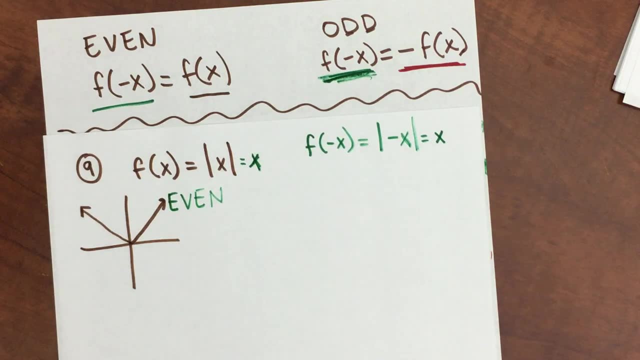 And this is the question that we are going to solve. graph. this is how it looks and when it has even symmetry, means that if you fold it, then this part will match the part on the left. okay, so it's perfect, because it does. if it, if it was not the 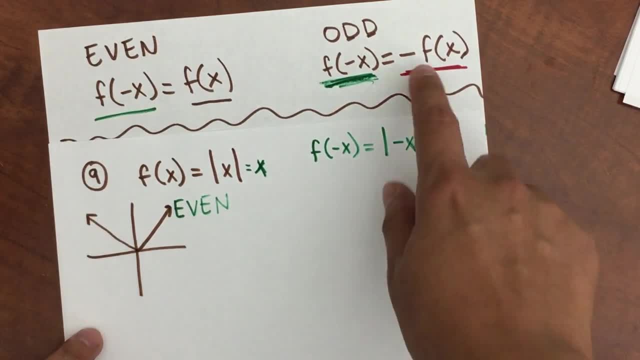 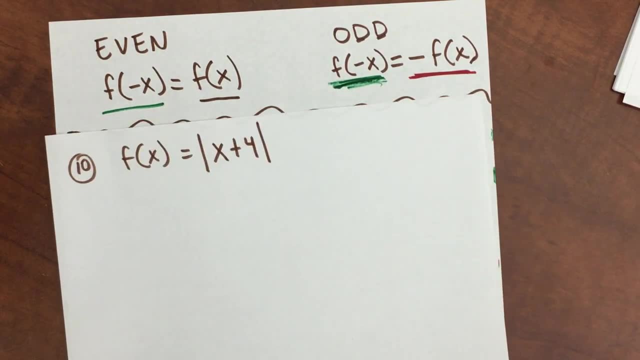 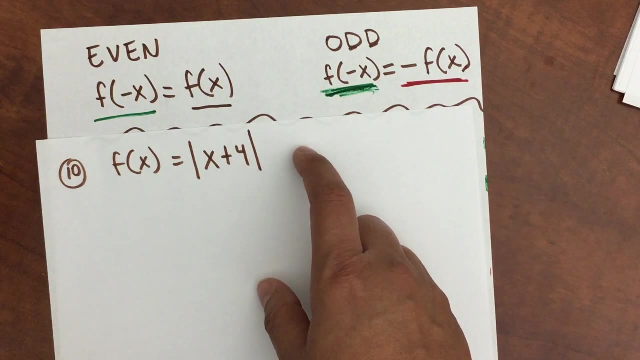 same, then that means that you would have to try the odd. so do the negative f of x. okay, so let's do another one. what if it's where you're adding something? so in here, basically we can, just we cannot say that you're always have positive x plus four because we don't know what the value. 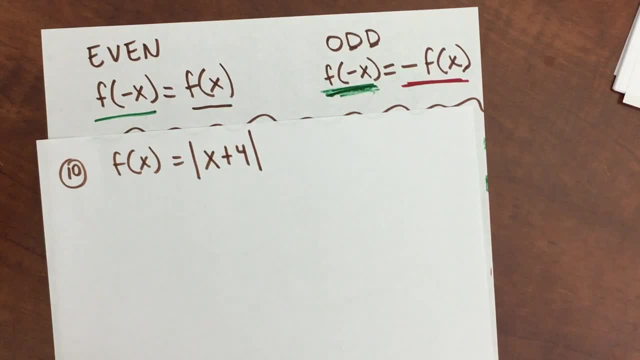 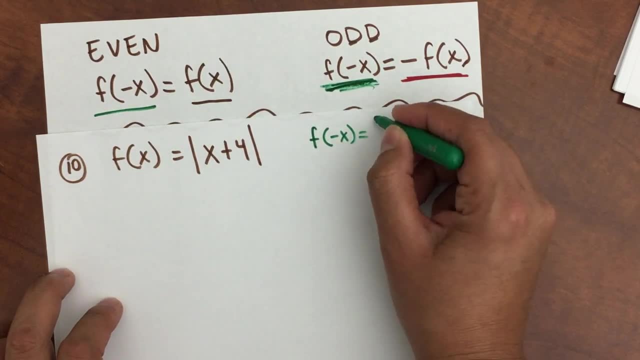 of x is. so we cannot simplify that, okay. and so f of negative x is equals to the absolute value of negative, meaning the opposite of what x is plus four. again, just because we're adding something in here, we cannot simplify that, we cannot automatically take it as. 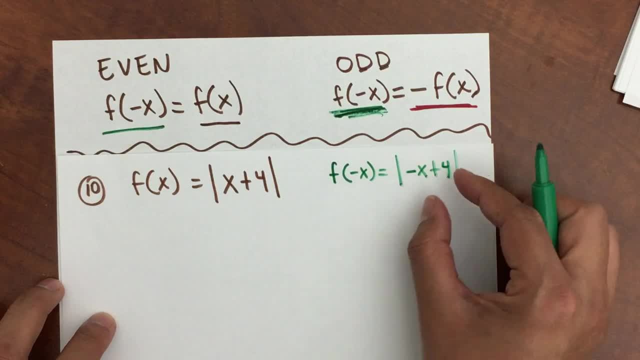 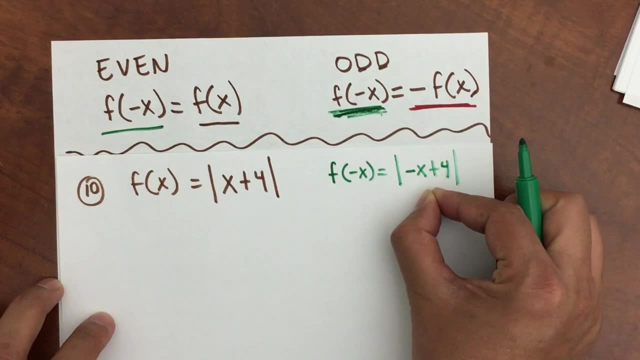 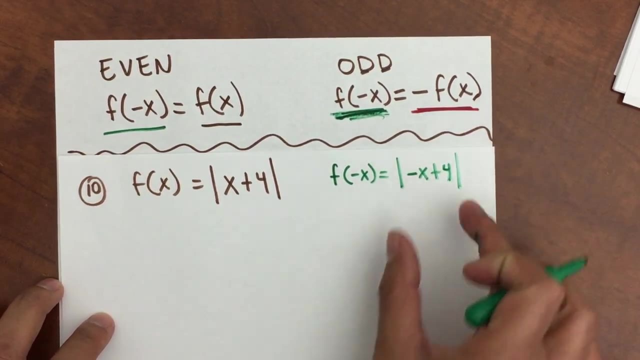 you, you, as positive, you always do the addition first, or multiplication, or whatever it's going on inside, and until you get one, one number, that's when you can take the absolute value of that number. so that's why, since we don't know the value of that, we cannot take it out, okay, so basically, this does: 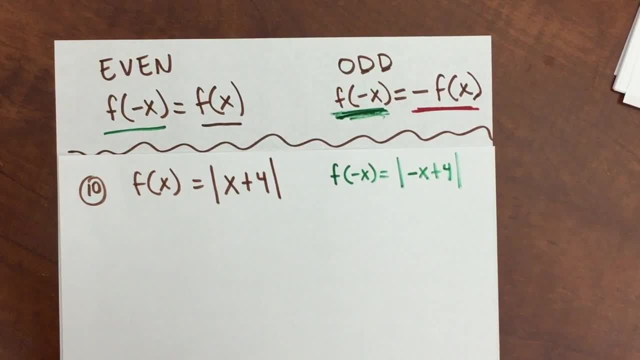 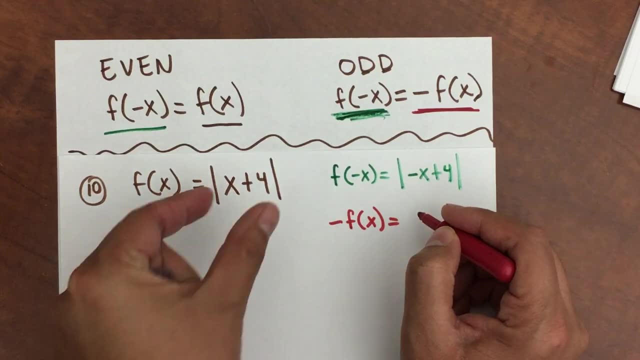 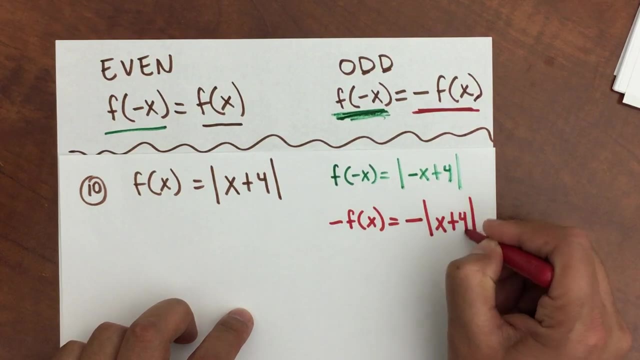 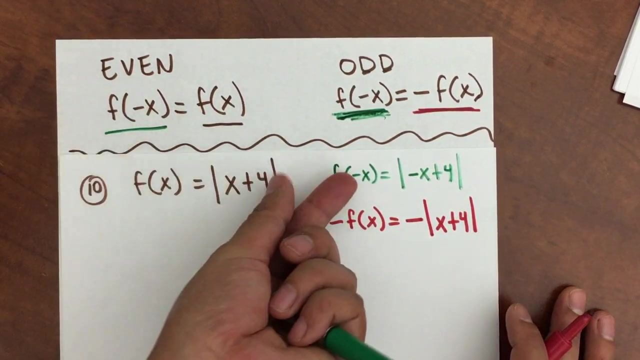 not look like this. so it's not going to be. uh, it's not even. then we're going to do the negative f of x, meaning take the opposite of that. so we're going to put a negative outside and the absolute value of x plus four. well, um, whatever answer we get in here, okay, whatever number we got, if we replace or substitute. 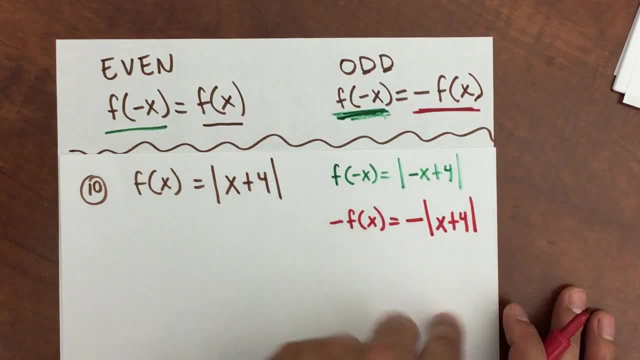 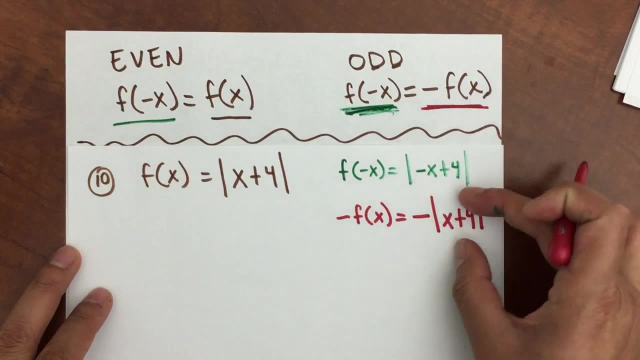 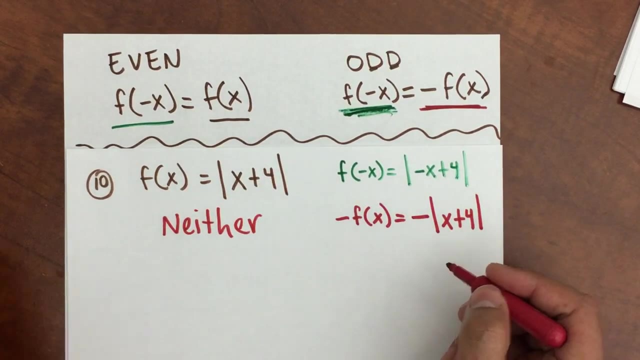 by values. that means that the answer in here will be the negative, and in here we don't have a match and so it's not going to be. they're not the same, so it's not odd. so we're going to say neither okay again for them to be. even this have to be the same for them to be. 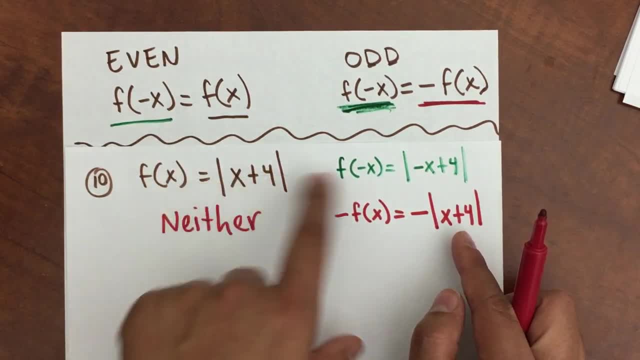 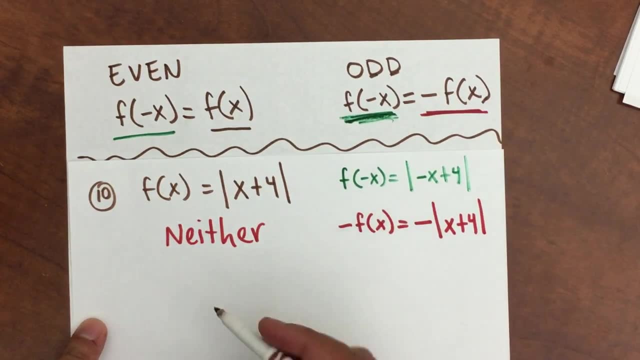 odd. for for the graph, for the function to be odd, then these have to be the same and they're not the same. so that's why we put neither. and if you look at the graph, let me sketch it. if you recall, the absolute value is the original goes in here, but then this goes to the 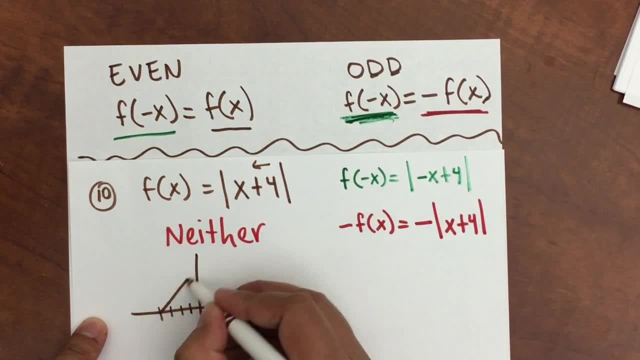 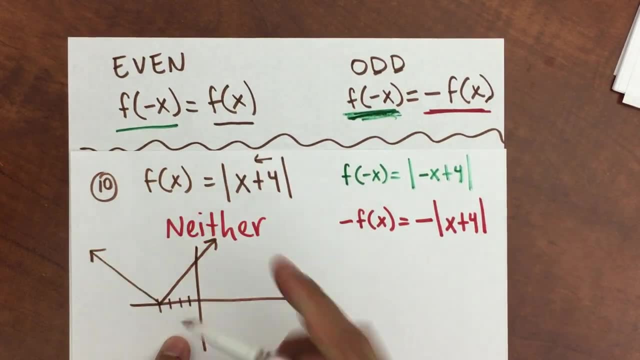 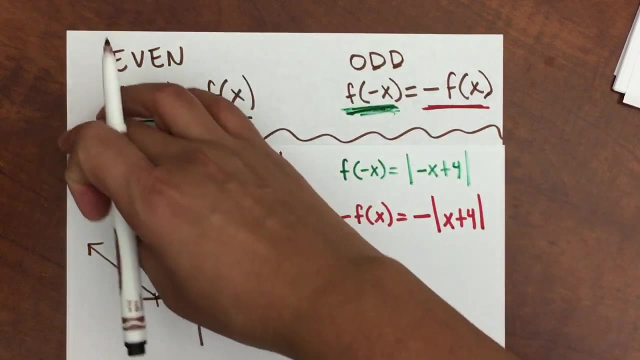 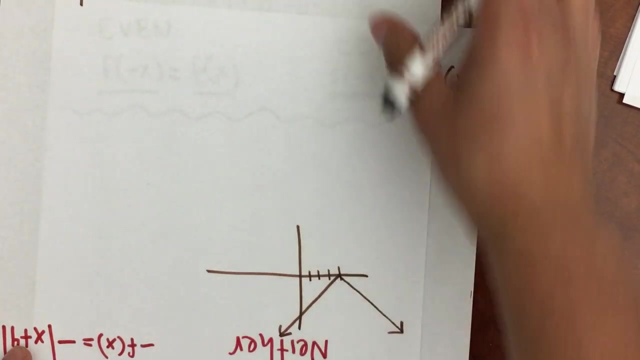 left four spaces. so it's going to be something like this: now, if you fold it along this line, fold it in here, you're just going to end up with something like that, okay. and if you rotate it 180 degrees, you don't get the same graph, because the original was here. this for this function. it was here, okay. 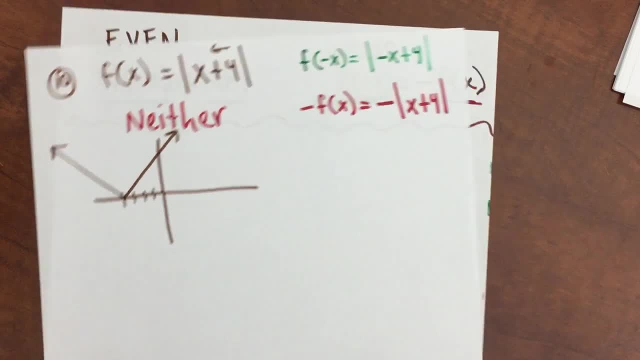 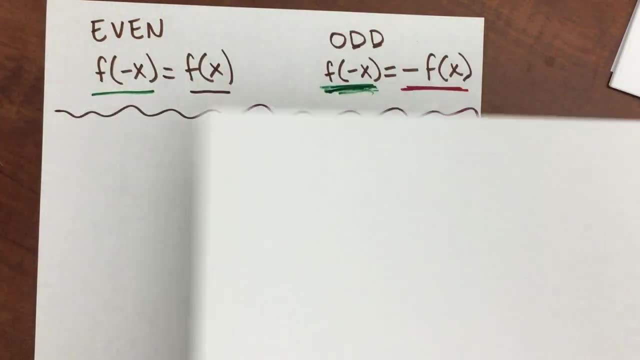 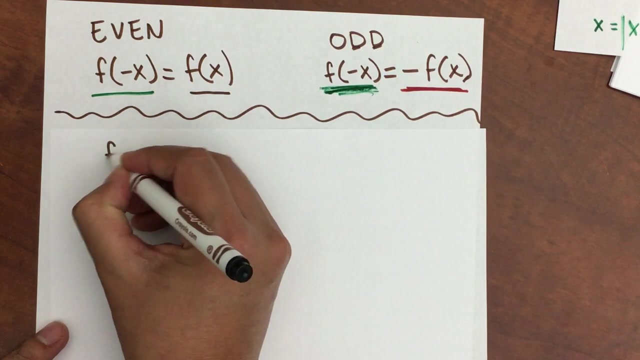 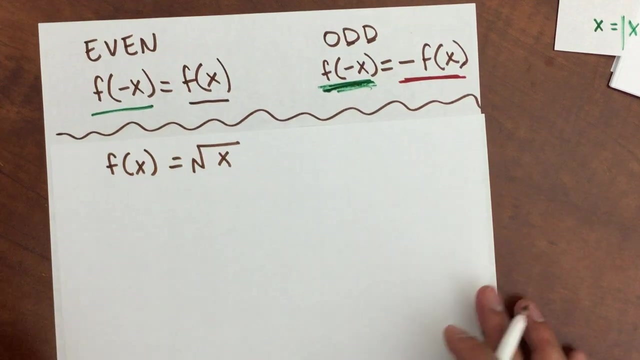 so that's why it's neither neither um, even, nor odd. okay, let me write another one. so let's do: f of x is equal to the absolute value of x, and this time i'm going to start with the graph. again, you don't have to do the graph, but uh, it's good if you recall the absolute value of x. 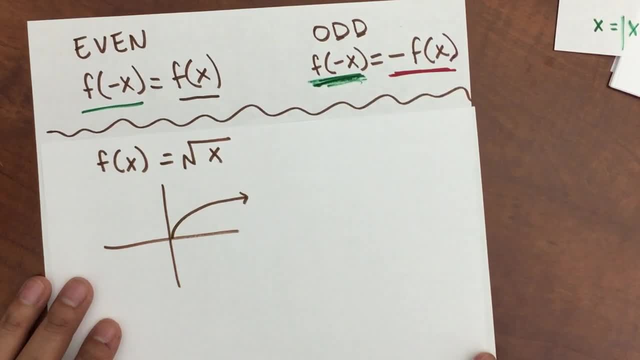 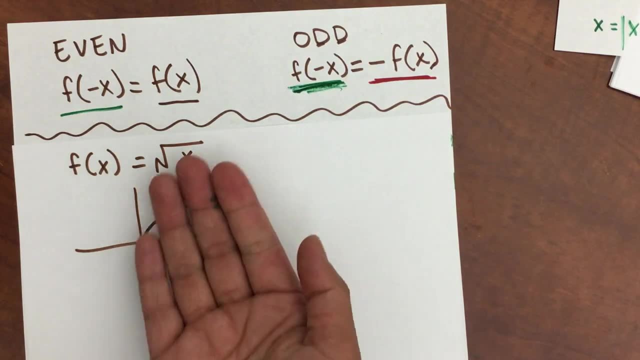 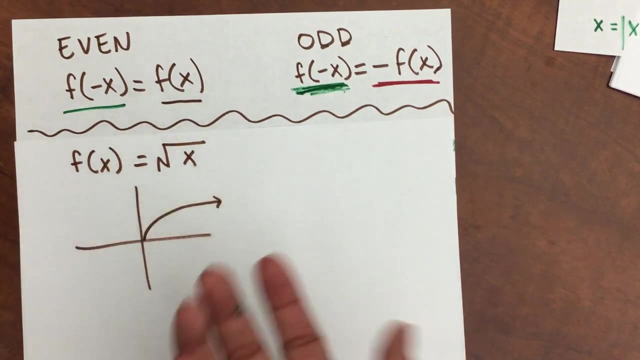 you just end up with something like this: okay, from previous lessons you just had to sketch to, and that's what you'll get. and so, algebraically, we notice that it doesn't match if you fold it, because there is nothing to match it with, and if you rotate it, you end up with something in here. so it doesn't match either. 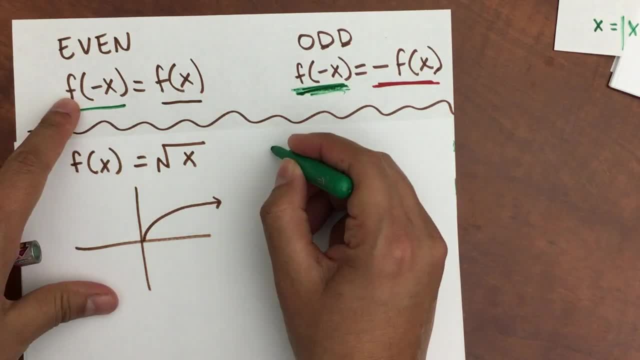 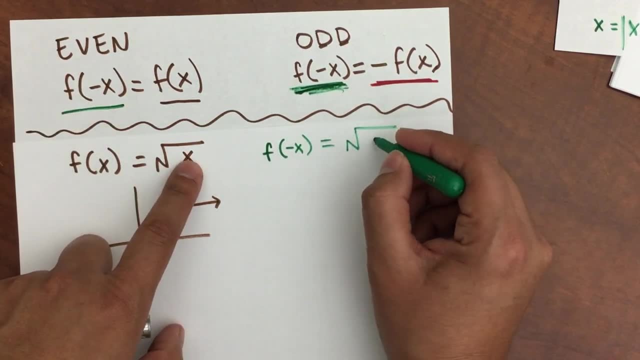 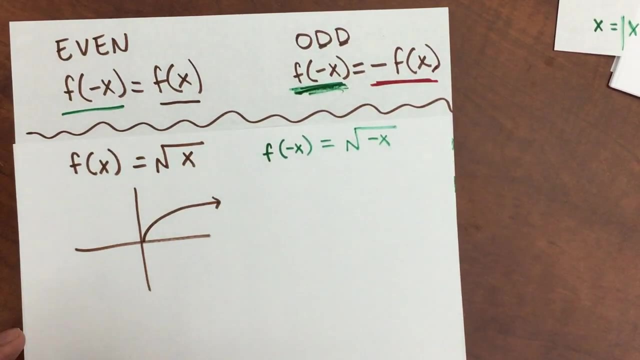 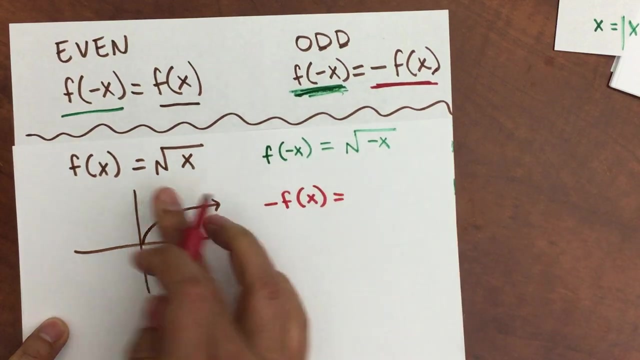 okay, but let me show you algebraically. you have f of negative. x is equal to the absolute value of, and now x is negative x. if you read well, it doesn't match, because one is positive, one is negative and you can add or- I don't like to simplify anymore now let's do the negative of f of x, meaning the opposite of this. 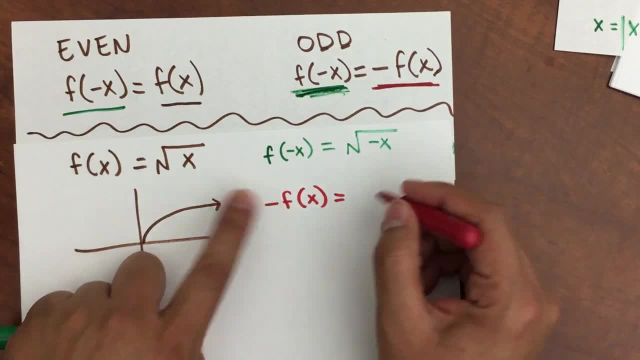 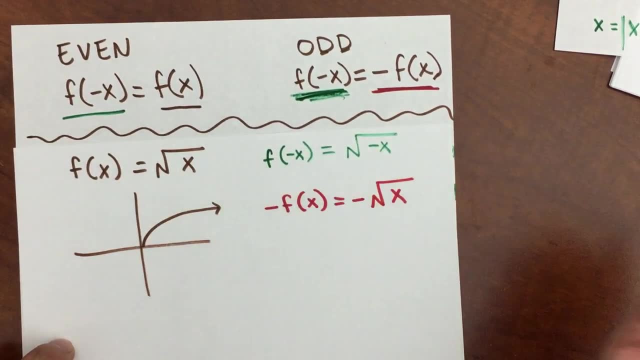 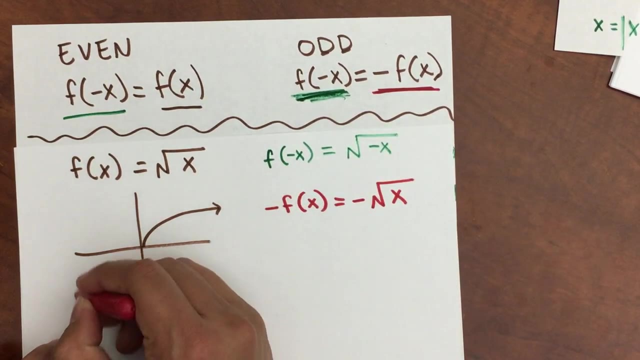 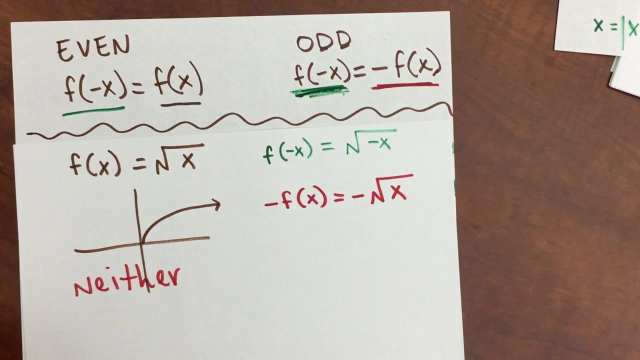 function right. get the function and multiply it by negative, so negative, and the function of x is square root of x. so these don't look the same. okay, this answer don't look the same, so therefore it's neither as well. now i'm going to show you, if you recall from previous lessons. this is just so that we understand why. 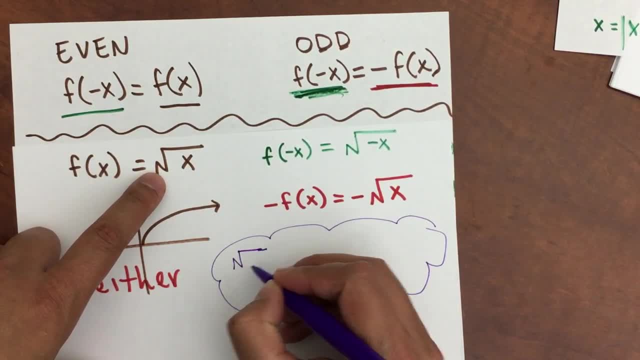 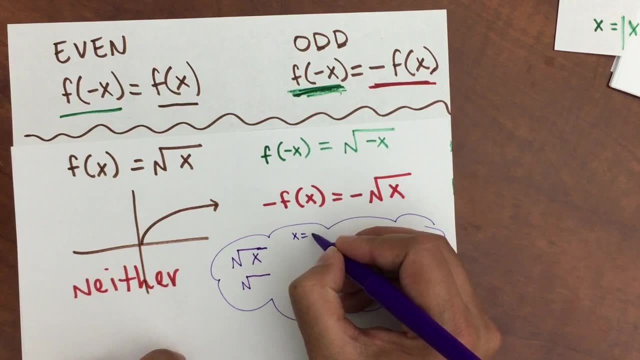 there are different, if you recall from previous lessons, the absolute value of x. let's say, just give value of x as 25, maybe. so the absolute, the square root, not the absolute value. I'm sorry, the square root of 25 is 5, because two numbers that multiply times itself equals 25. well, that will be 5 now for. 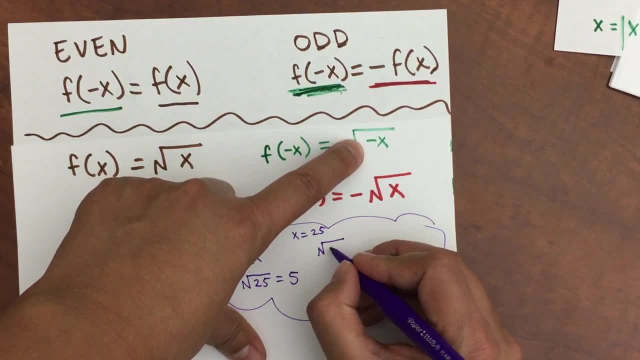 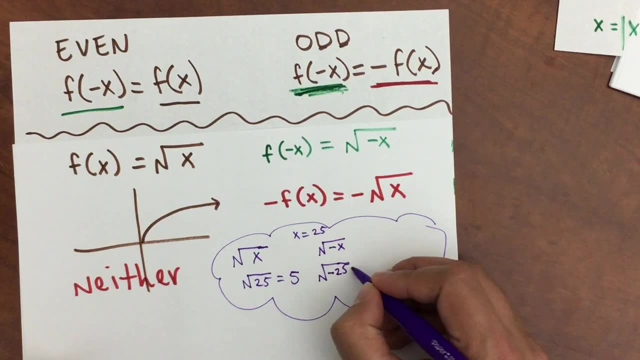 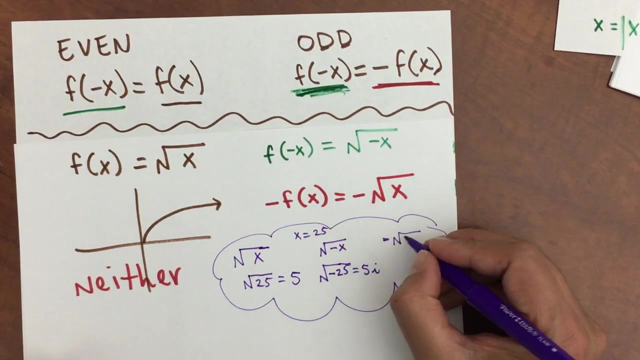 this one. you were talking about the absolute, the square root of negative x, then we put negative 25 and, if you remember, the square root of a negative becomes I, and then square root of 25 is 5 and the negative. okay, now I'm doing this part- the negative. 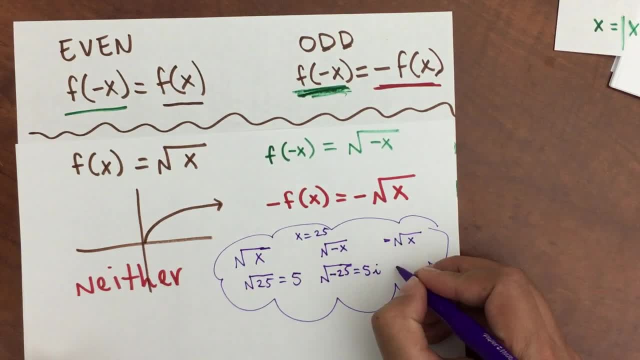 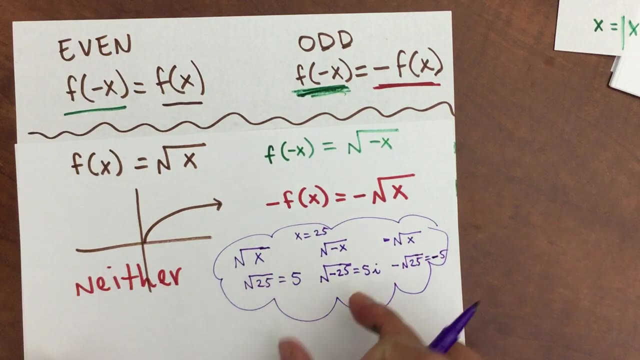 square root of x, then let's do negative square root of 25, if you recall this, because it's outside, you just bring it. sorry about that. and the square root of 25 is 5. so this is this. it's not the same as this, right? they're not the same. 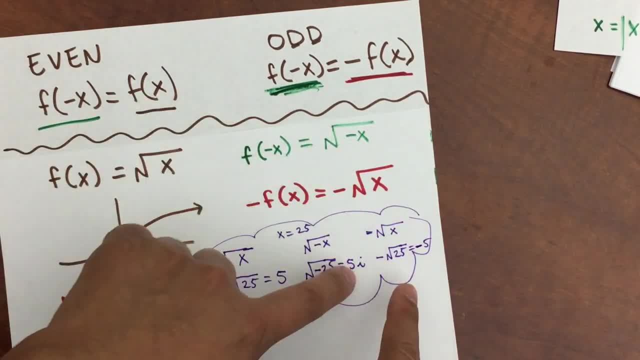 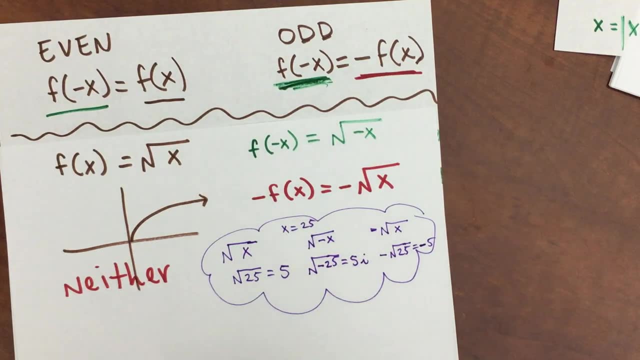 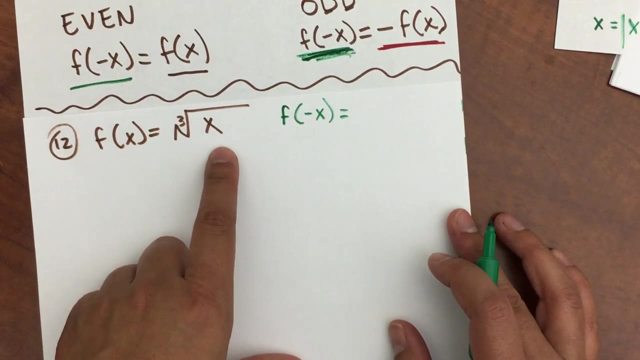 so it's not even and this is not the same. so for this one it will be this one, and this will be the next one example of this one. they're not the same, so therefore is not odd either. so in here this one is tricky, and the reason is because for the square root, you cannot. 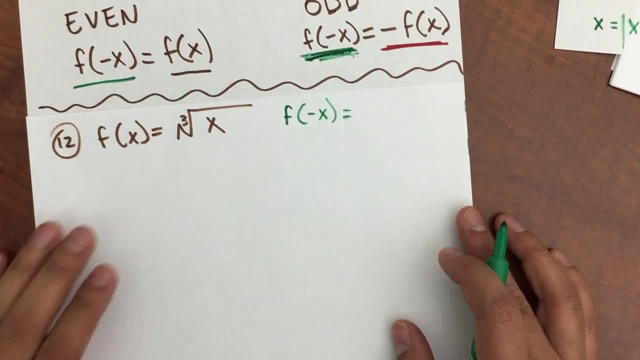 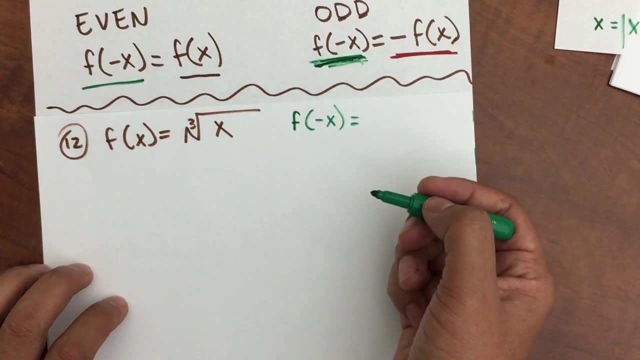 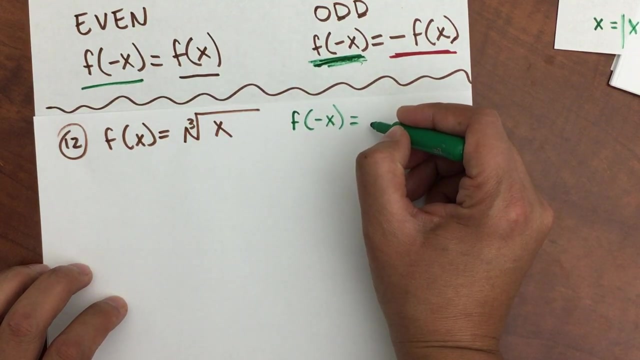 have a negative inside or otherwise, it becomes an imaginary number. but this cubic root. what it means is that you're looking for a number that multiply, times itself. two, three times, yeah, three times is equals to the number in inside, and so in here you are able to get answers for negatives. for example, if 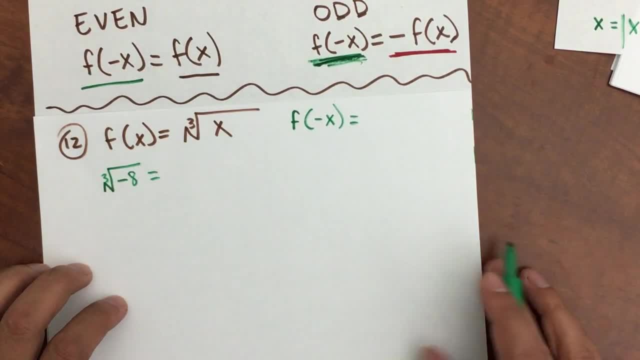 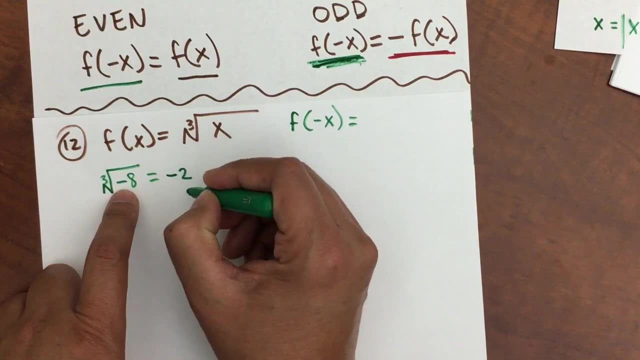 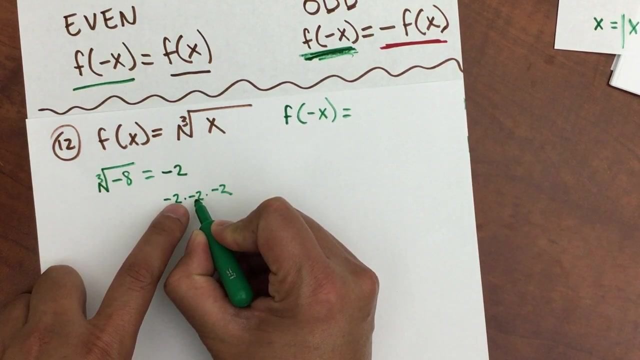 you have the square root of negative, the cubic root of negative: 8, a number that multiply, times itself three times and equals negative 8 is negative 2. why? because negative 2 times negative, 2 times negative, 2 negative times negative, positive and positive times negative. negative 2 times 2 times 2- 8. so 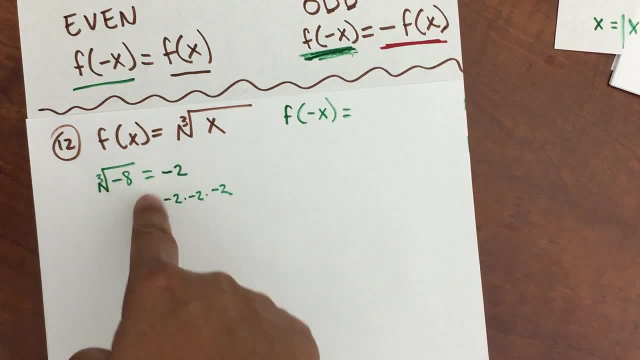 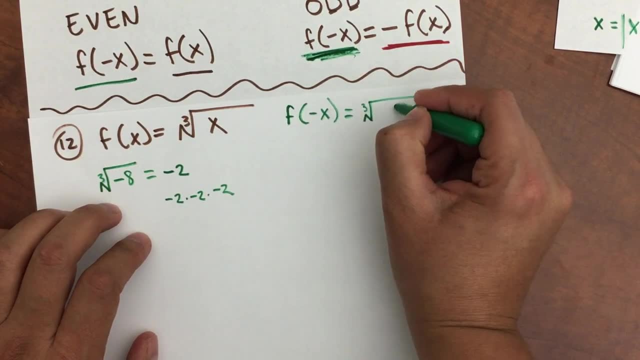 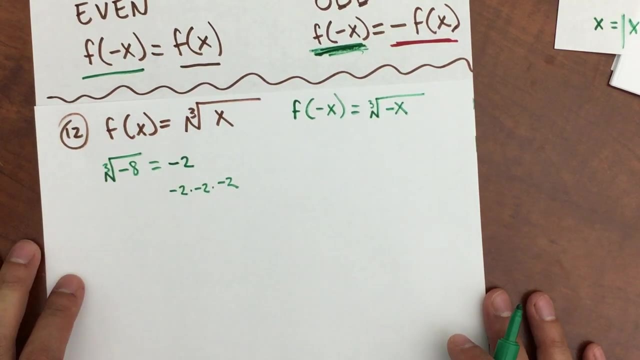 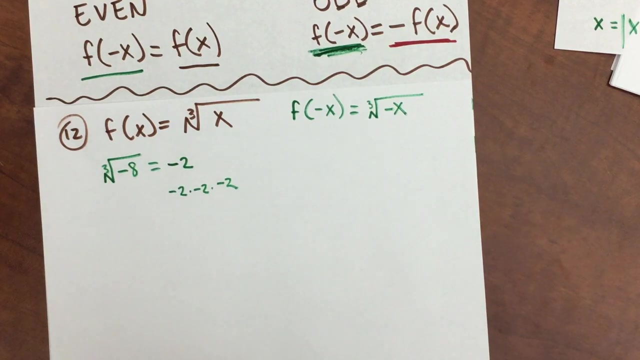 you are able to actually get the cubic root of a negative number, ok, and so in here we're going to have the cubic root of negative x and we say that they look the same. well, one thing that I also showed was by doing kind of like a test where, or by 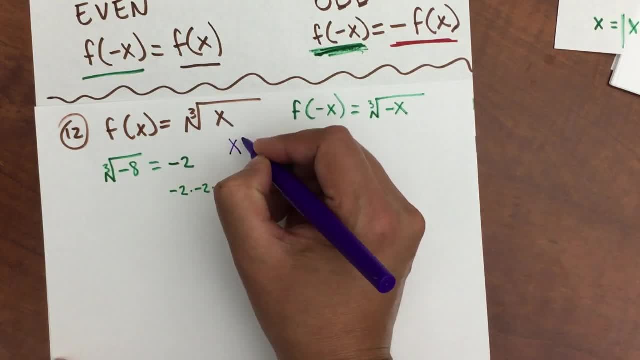 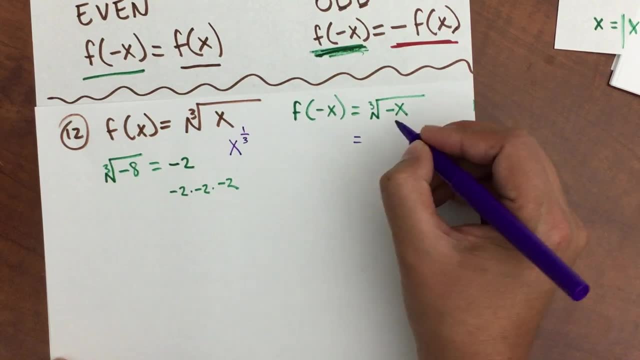 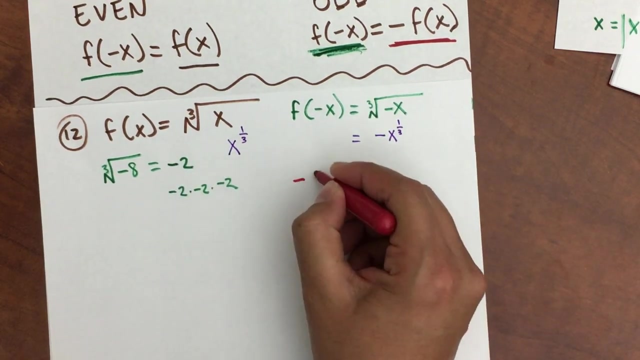 putting the X. remember that this exponent becomes the numerator and the index becomes the denominator. and in here you will have negative X. this becomes the numerator, this becomes a denominator. ok, so they don't look the same. now the negative F of X is equals to: we put the negative and then 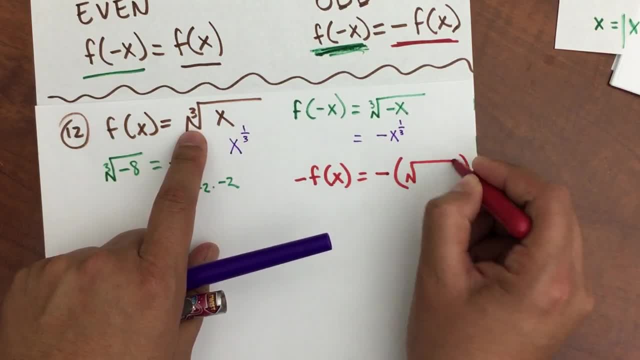 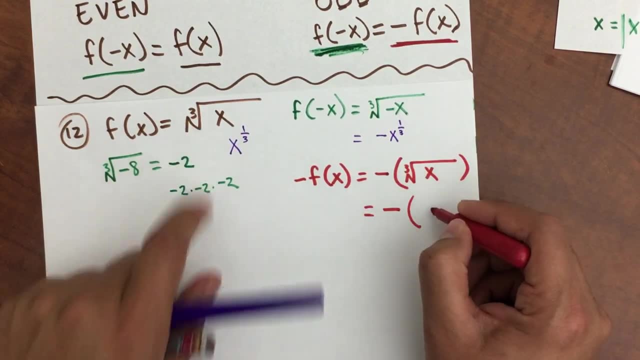 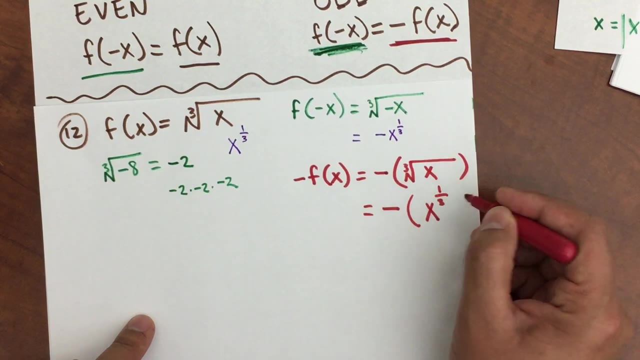 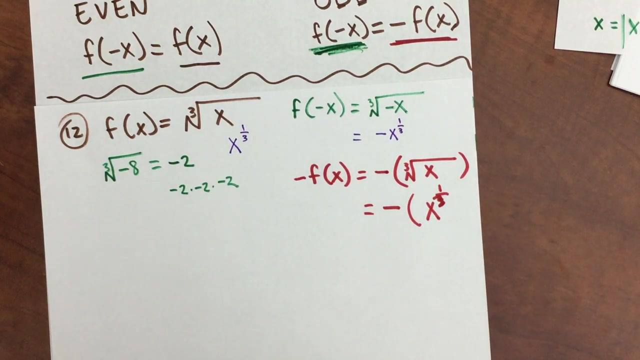 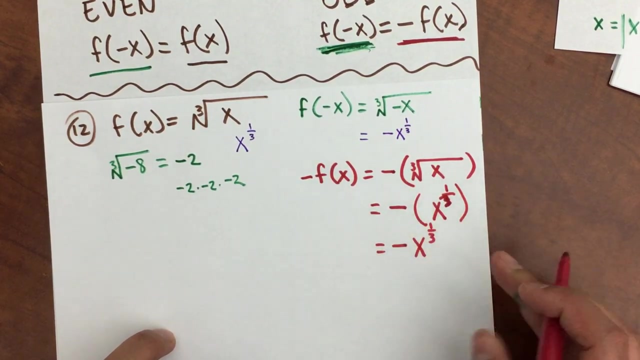 side. we put the original function, which is cubic root of X, we put the negative and we rewrite this as X. the exponent becomes the numerator, the index becomes the denominator. ok, and so when we multiply this negative times positive, it becomes negative. and then we have negative x divided by the minus, x valued by the division of x one to the 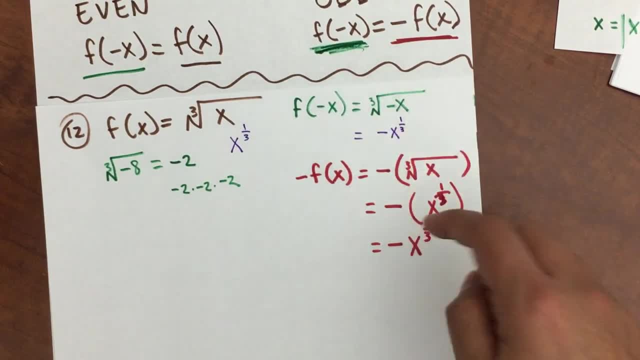 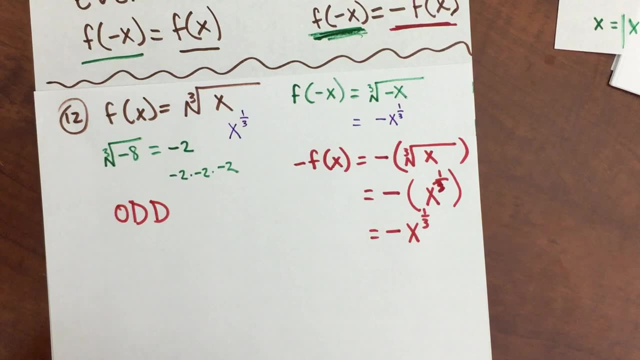 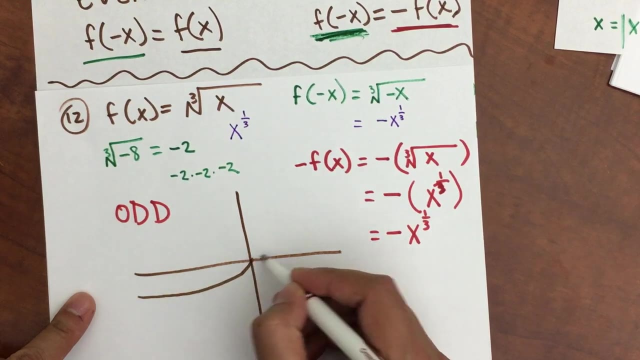 third- so this is from another lesson, also converting from roots to rational exponents, and it's easier to compare this because you can see that they are the same, and so we can say that this is odd. the graph, the sketch for this will be something like this: 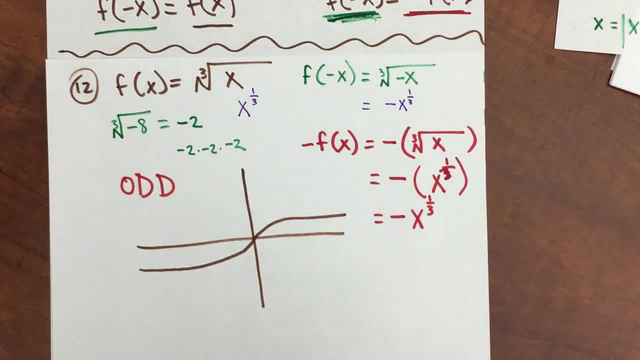 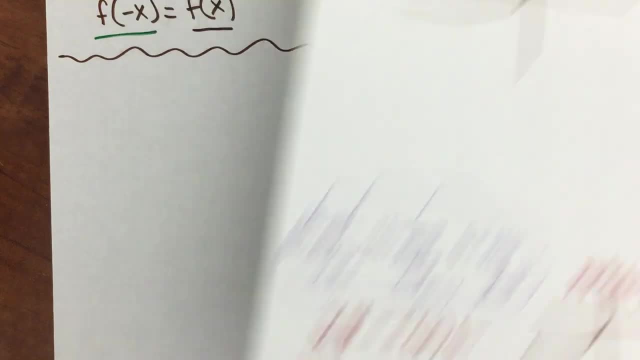 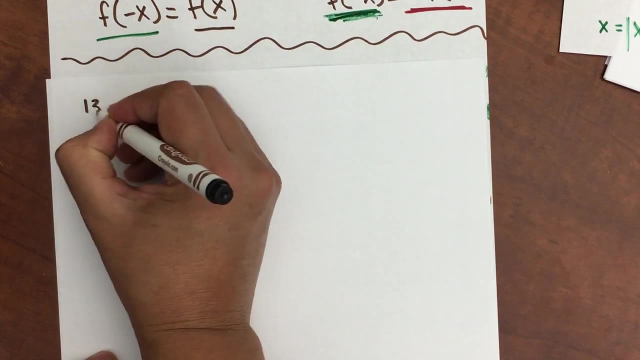 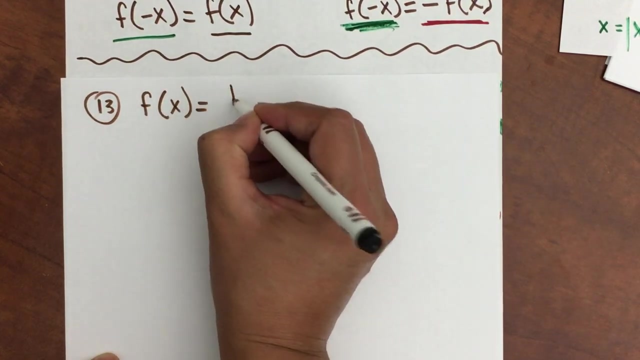 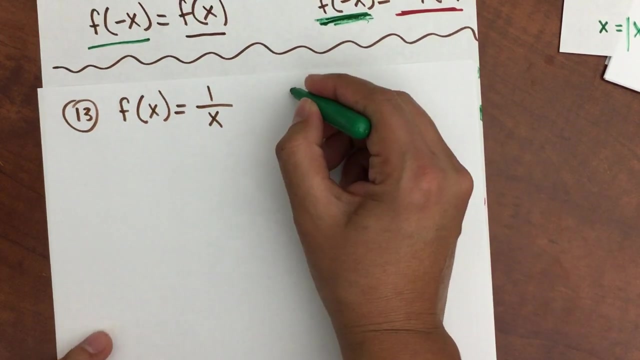 you flip it, you end up with the same. if you flip it, if you rotate it 180 degrees, then you will get the same answer once again. while I write the other one, I would like to apologize for the announcement there. okay, number 13, and so it's gonna be: f of X is equals to 1 over X, and I put f of negative X. you put the.